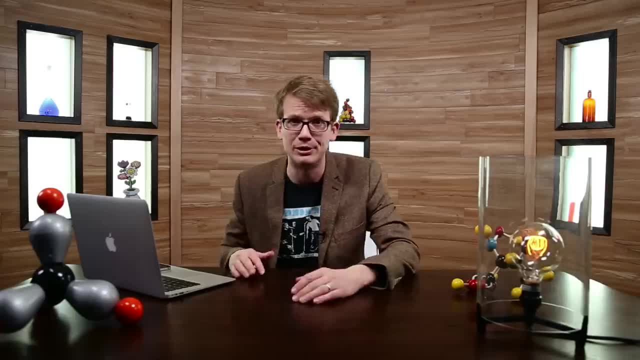 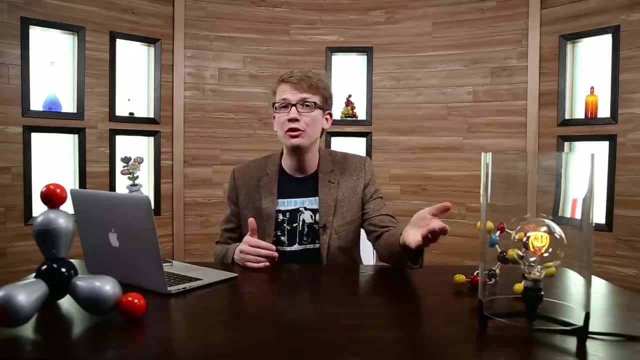 in a committed relationship or you're married. There are all kinds of different combinations of people out there And sometimes you know people fall for a vampire or a werewolf. Who am I to judge? Fact is, each type of relationship requires different things from you and the 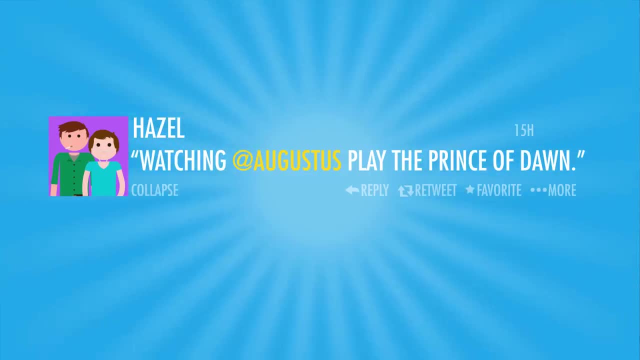 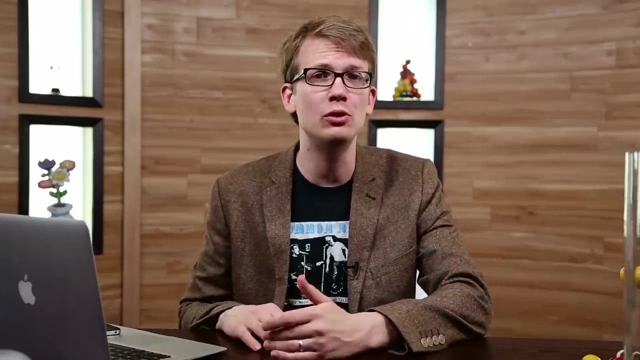 other person. But if you play your cards right, these relationships allow you to relax and escape the stresses that come with the constant search for affection. Distance is important in relationships too. Of course, too much distance makes it hard to stay focused on each other and requires a lot of effort to keep things together And 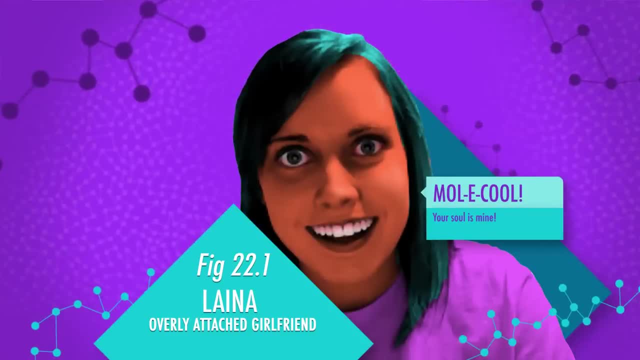 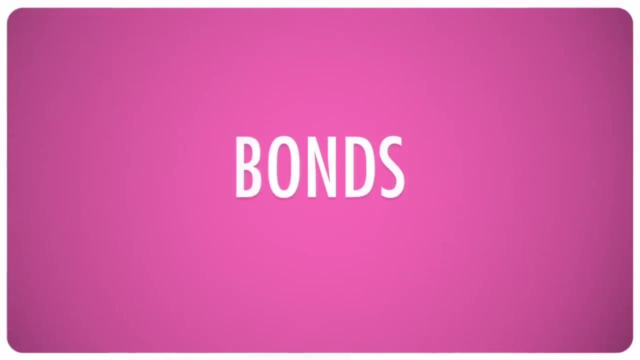 I may not have to tell you, too little distance can be a problem as well. Everyone needs their space, and when you don't have any, you just end up pushing away from whatever's crowding you. In this way, atoms are a lot like us. We call their relationships bonds, just like. 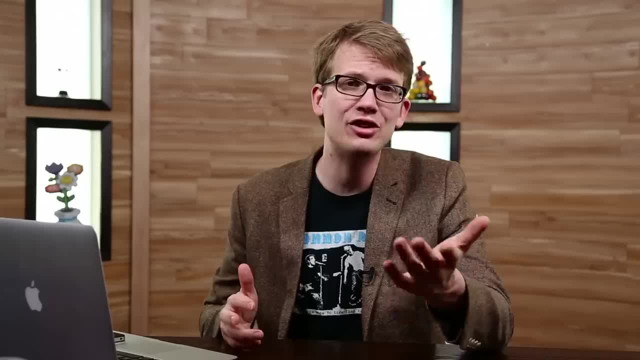 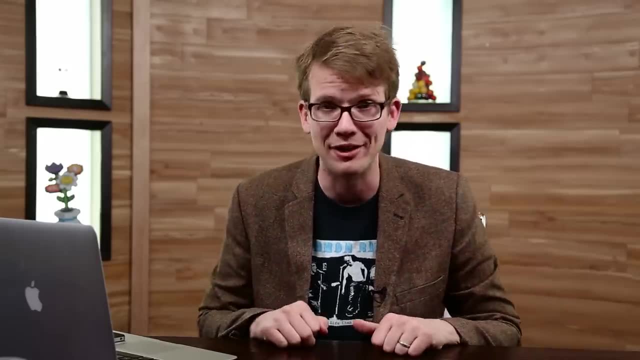 we do with our own relationships, And there are many different types. Each kind of atomic relationship requires a different type of energy, But they all do best when they settle into the lowest stress situation possible. The nature of the bond between atoms is related to the distance between them And, like people, 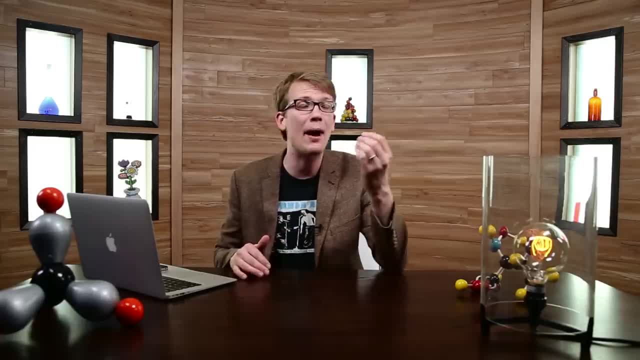 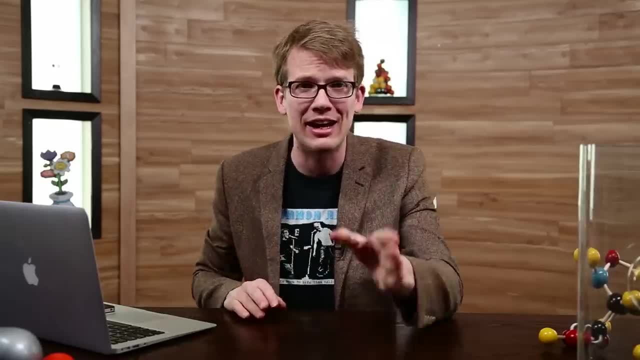 and vampires and werewolves. I suppose it also depends on how positive or negative they are. The difference is that, unlike human relationships, we can analyze exactly what makes different kinds of chemical relationships work, And that's what this episode is all. 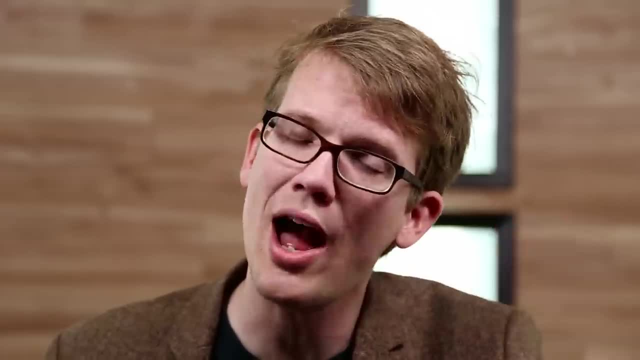 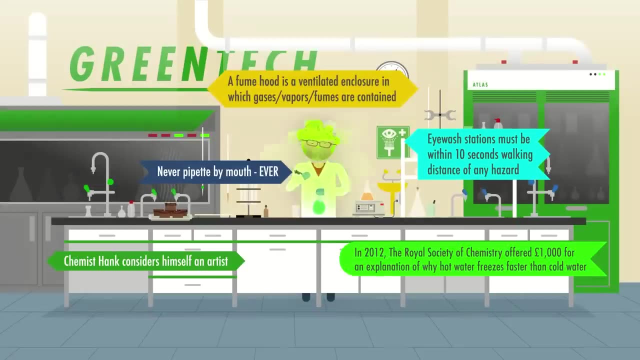 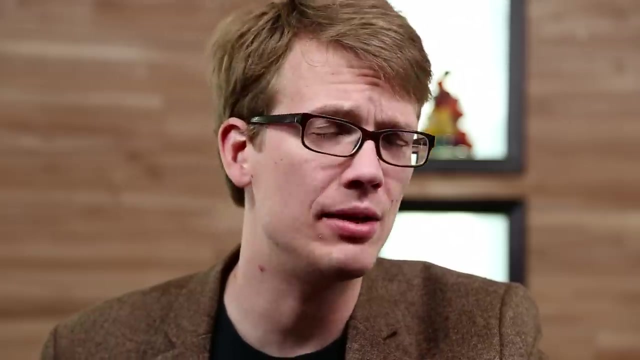 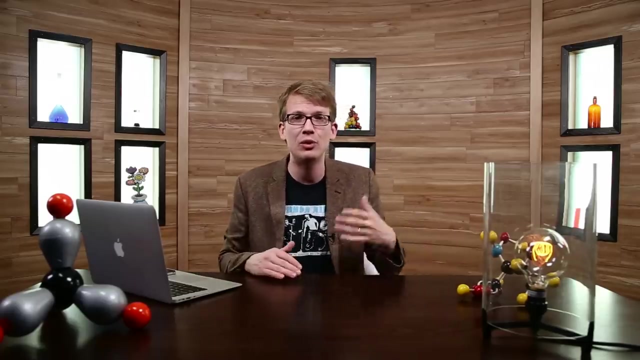 about. But people, please remember that we here at Crash Course do not dispense relationship advice. First things first. why do atoms do this at all? Well, like everything else in the universe, atoms do whatever they can to reduce their overall energy, And they reach their 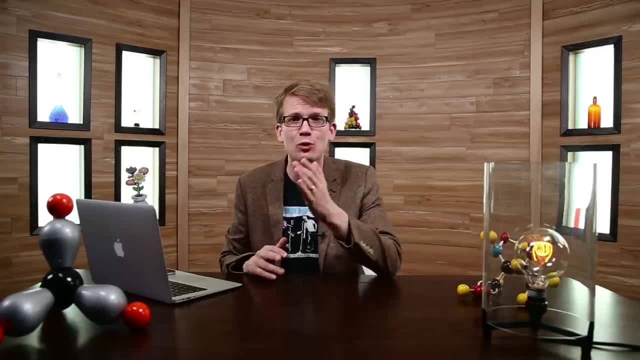 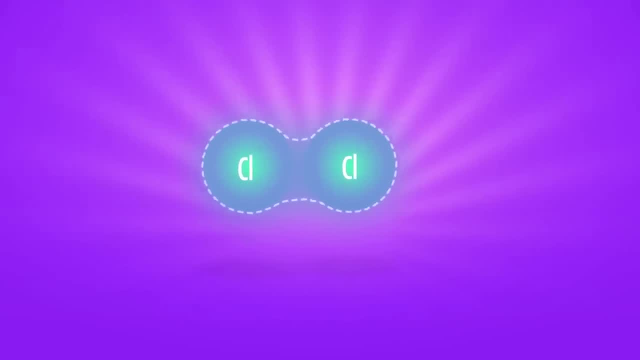 lowest energy by achieving a balance between attractive and repulsive forces, being neither too clingy nor too aloof. So when two atoms approach each other, the electrons of each are attracted to the protons of the other. This is the electrostatic force, Like charges. 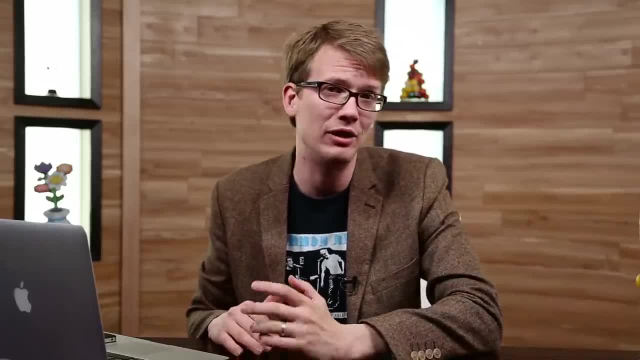 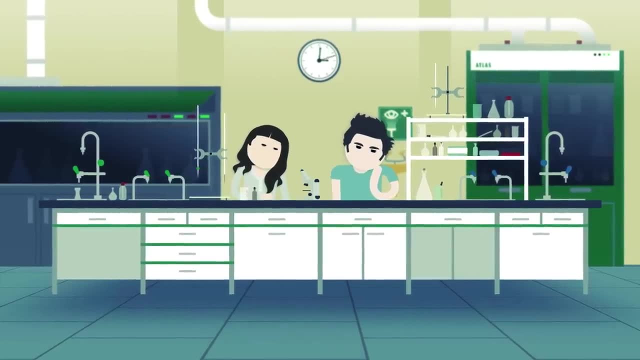 repel. opposites attract, Like in real life, or at least Paula Abdul songs. I know I'm old. So when one atom is attracted to another- just like Edward Cullen and Bella in chemistry class, to use a slightly more timely reference- it gets stressed out by the attractive force. 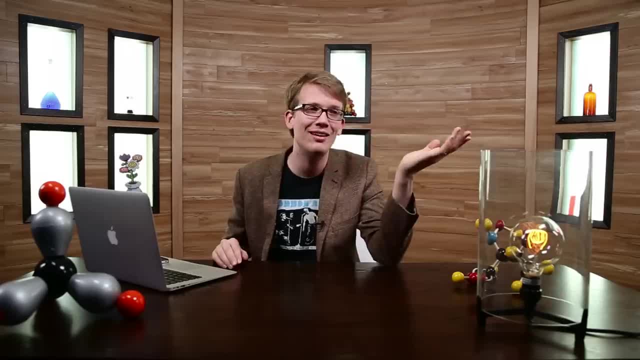 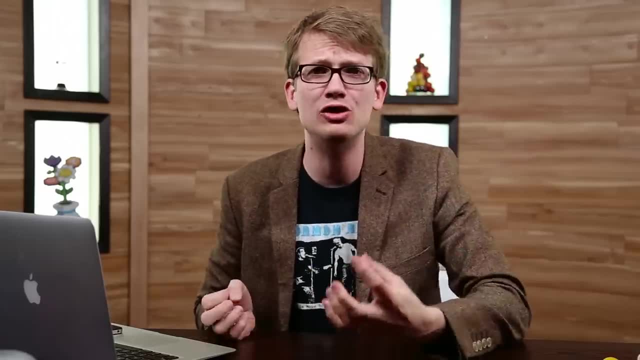 and tries to relieve the stress by getting closer. We've all been there, right? That hot, nerdy vampire girl in your chemistry class. It's just, it's intense. They're both so strong that the stress level, or energy, rises when the two are separated. so they stay close, But sometimes they can get a little too close. When that happens, the nuclei repel each other because of their like charges and the energy between them rapidly increases and they both back off just enough to find that perfect little distance. 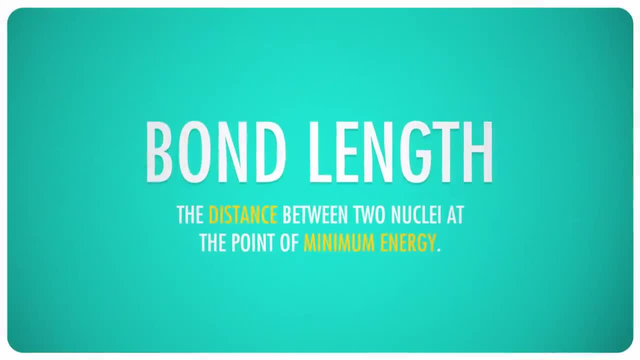 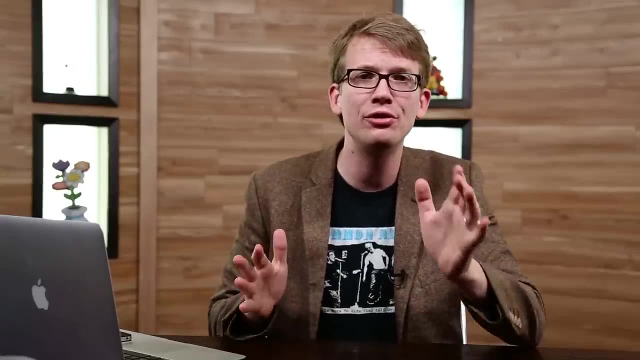 between them and everyone relaxes. This ideal, wonderful distance is the bond length. It's the distance between two nuclei at the point of minimum energy, In other words, where the attractive and repulsive forces cancel each other out. The distance at which these two atoms of chlorine reach their minimum energy, caught between 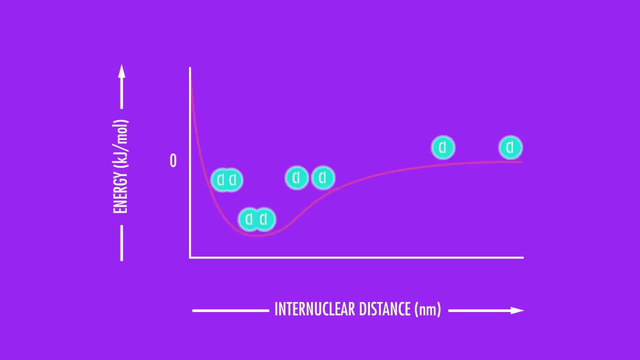 the attraction of the electrons to the nucleus and the protons. repelling the nuclei is the bond length, That energy minimum, which we know absolutely is negative two hundred and thirty nine kilojoules per mole, occurs when the distance between the atoms is zero point. 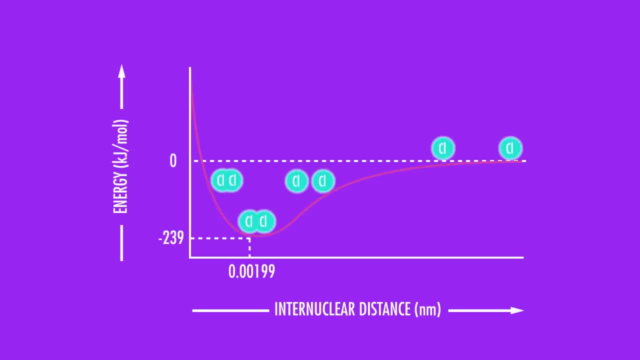 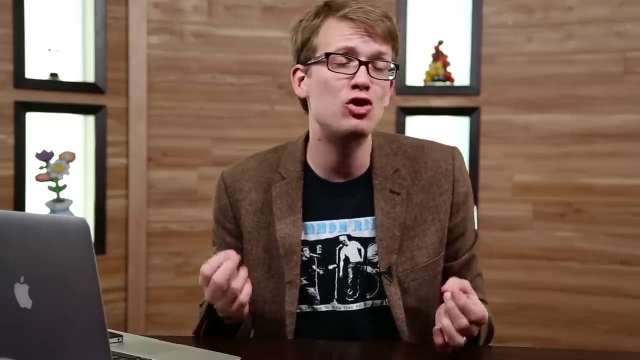 zero, zero one, nine, nine nanometers. That distance is the bond length of Cl2, chlorine gas. Now, because the electrons are attracted to both nuclei in the molecule, they actually spend the majority of their time in the space between them. The bond length is often described as sharing electrons, and we call this kind of bond a 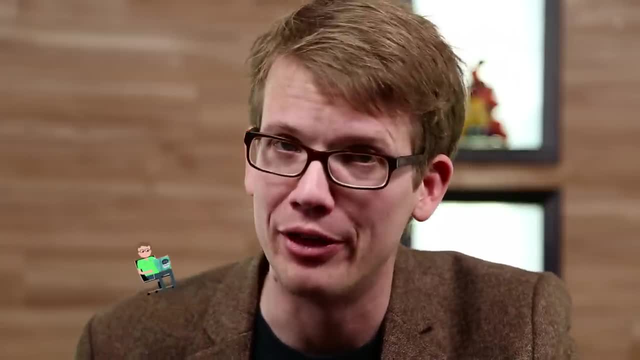 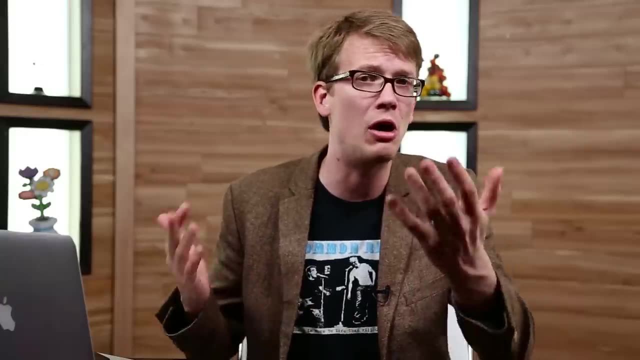 covalent bond. But not all sharing is equal. I should know I have an older brother. The strength with which an atom holds shared electrons is called its electronegativity. The electronegativity is that various elements are all super well known and waiting for you. 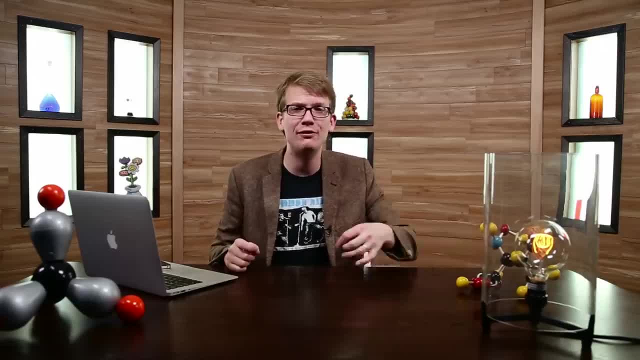 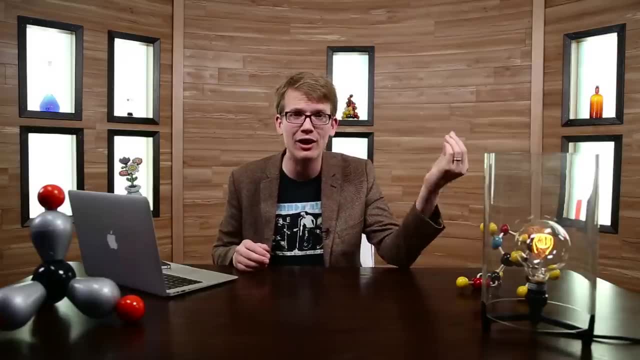 in tables on the internet. If two atoms in a bond have very different electronegativities, like say hydrogen at two point one and oxygen at three point five, the electrons are more attracted to the atom with the higher electronegativity. The difference is so great that the electrons spend the most. 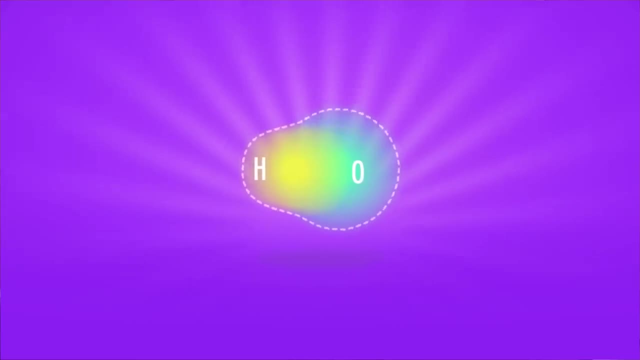 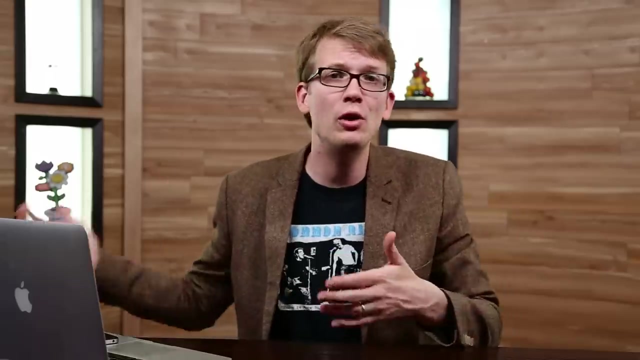 of their time around the stronger atom and much less time around the other one, like how all the neighborhood kids wanted to hang out with John, my older brother, because he was more charismatic. When the electrons hang out closer to one side of the bond, it creates a slight negative. 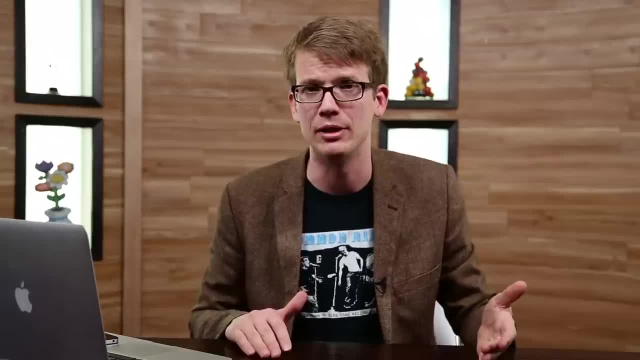 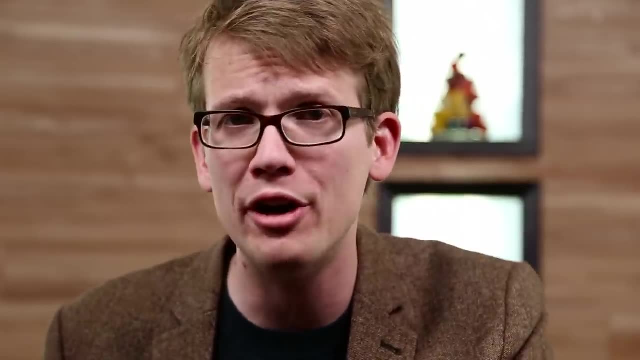 charge in that area and a slight positive charge around the other atom. This separation of charges is called polarity, and it's the polarity of the molecule that these atoms form- H2O- that makes water the most important molecule on Earth. Covalent bonds like this, where electrons are attracted to one atom more than the other. 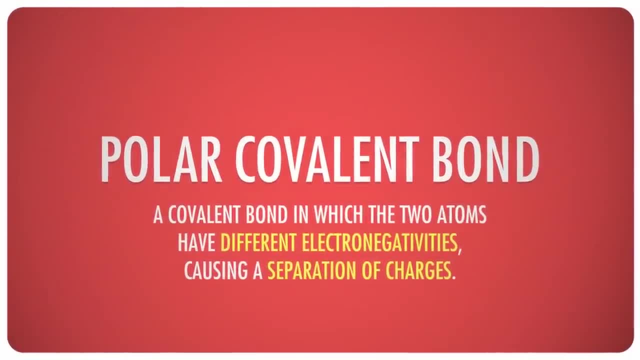 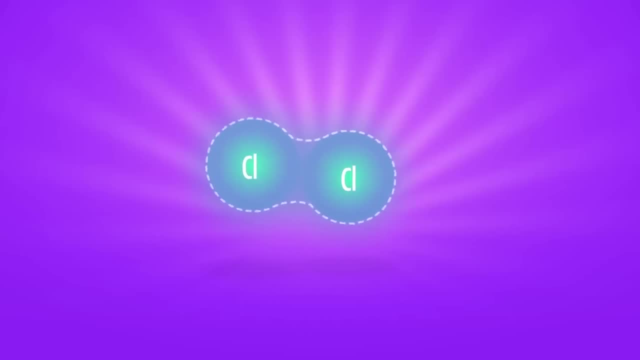 causing a separation of charges are called polar covalent bonds. But when a covalent bond forms between two identical atoms, like the two chlorine atoms in our graph earlier, the electrons are distributed evenly. We call this a nonpolar covalent bond. 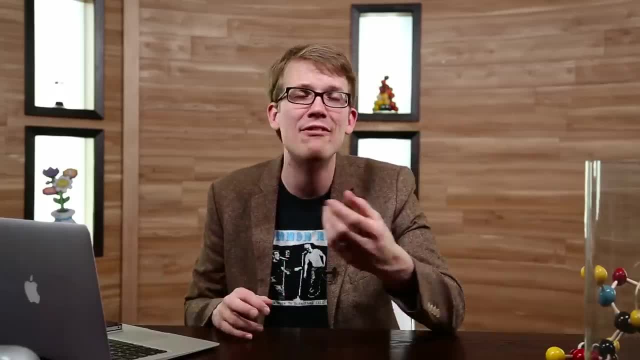 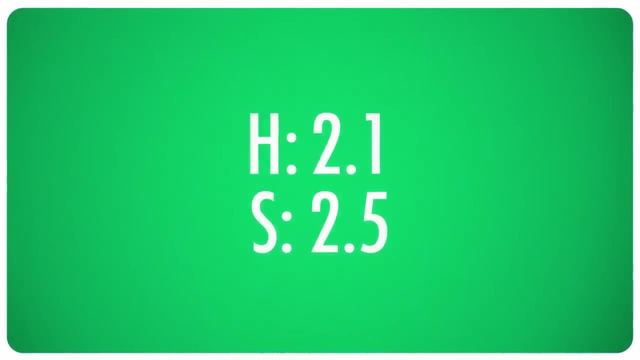 But you've also got to consider the middle option, where the atoms aren't identical but have very similar electronegativities, like hydrogen with an electronegativity of two point one, and sulfur at two point five. The difference here is so tiny that the electrons 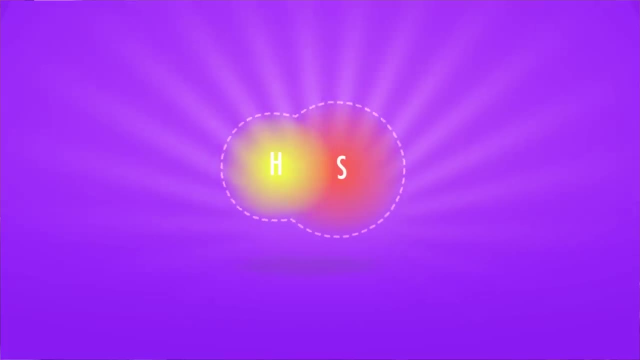 are pretty much still evenly distributed and we call that a nonpolar covalent bond. Now let's take a look at the nonpolar covalent bond. There's a huge world of important chemicals that have these kinds of bonds- so many in. 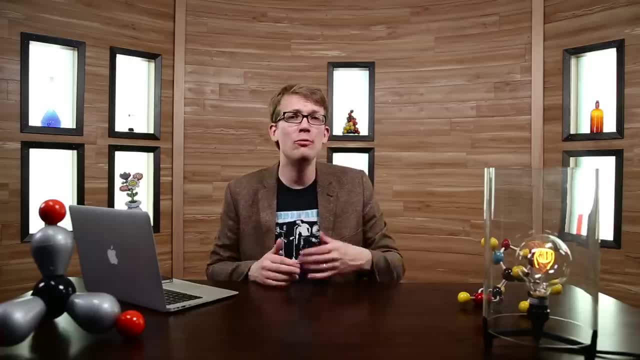 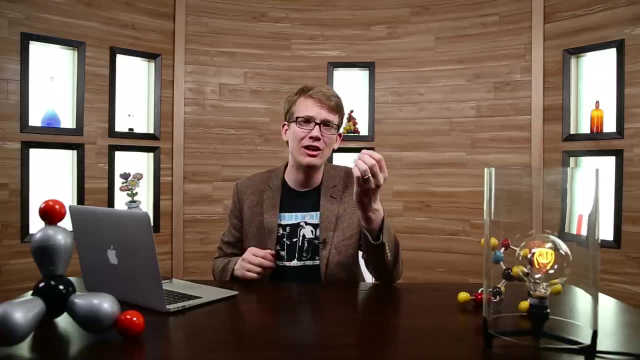 fact that we will dedicate a couple of separate episodes to them. Covalent bonds tend to form from nonmetals and sometimes metalloids, those elements that have both metallic and nonmetallic characteristics. That's because most of them hold their electrons. 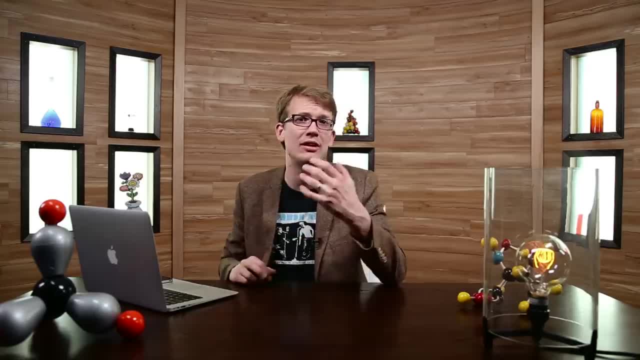 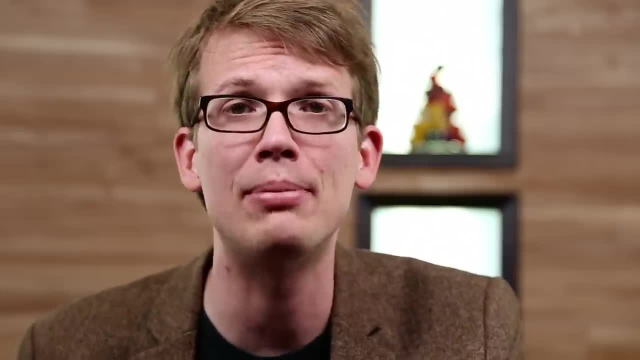 so tightly that they're more likely to share them with another atom than to gain or lose them altogether. Metals, on the other hand, have loosely held outer electron shells, so they're constantly dropping electrons and becoming positive ions, And when positive ions come across, negative. 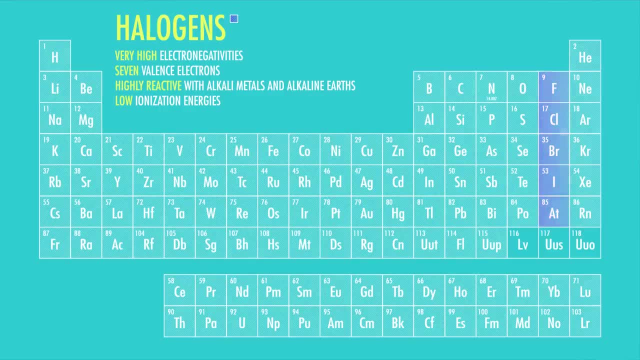 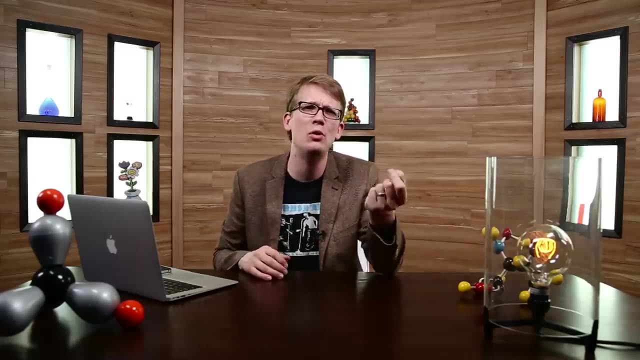 ions like those formed from halogens, for instance, you have to know what's gonna happen. They're attracted to each other, which means energy is required to keep them apart, which means that they're gonna bond if they can, creating that oh-so-wonderful point of. 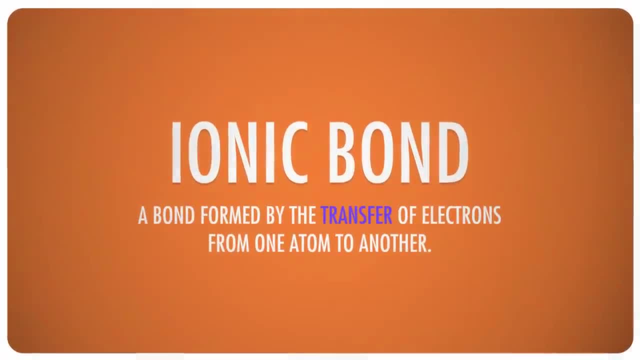 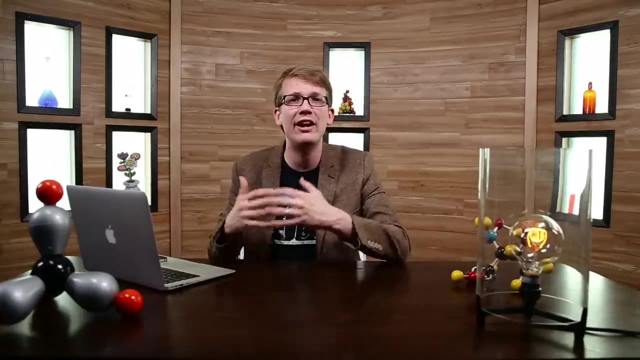 minimum energy. This type of bond is unsurprisingly called an ionic bond, a bond formed between a positive ion and a negative ion, Because the ions are formed when one atom loses electrons and the other gains them. we often say that an ionic bond is formed by the transfer of electrons. 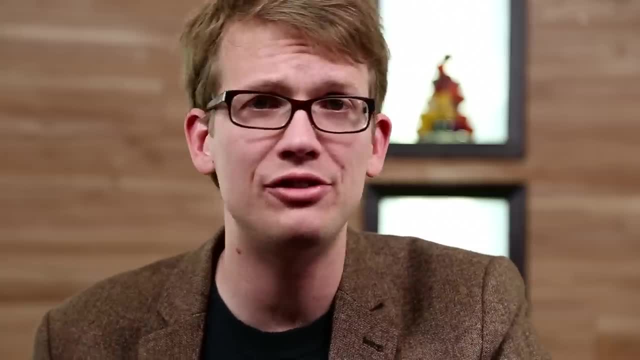 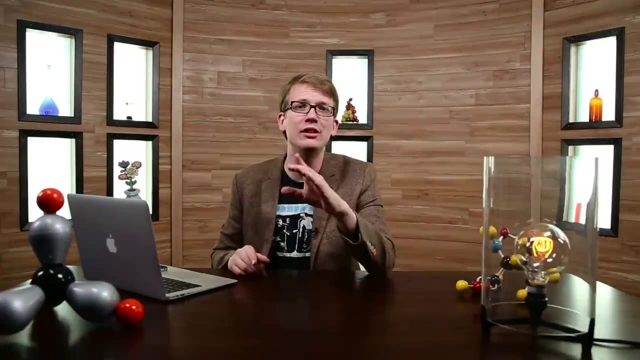 from one atom to another And we can calculate the amount of energy that exists in a bond between ions at a given distance using a formula called Coulomb's Law. Note that this only works for ionic bonds, because the calculation requires the charges of the ions which covalent bonds don't have. 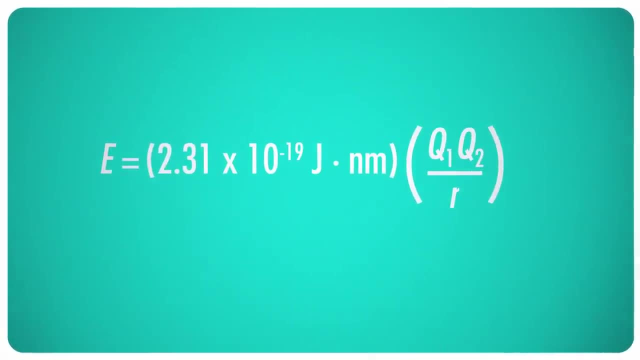 Coulomb's Law says that the energy between two ions equals the product of the two charges, which are represented by capital Qs. because why not? divided by the distance or radius between the two nuclei, all multiplied by a constant 2.31 times 10 to the negative 19th joules per nanometer. Of course, the radius also. 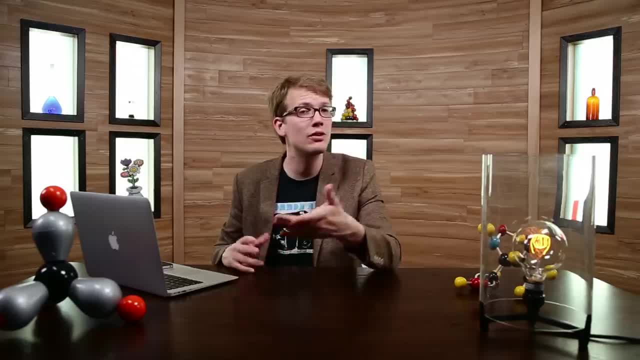 has to be expressed in nanometers, even though it's not a constant, But it's a constant, so you've got to make the units match. Let's see how it works with something simple: sodium chloride or table salt. We know that. 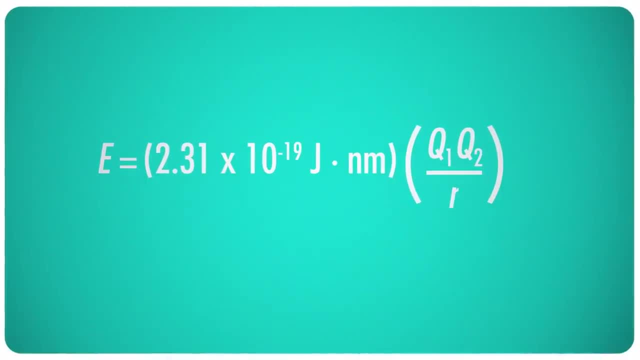 the normal charge on sodium ion is plus one and the normal charge on chloride is negative one. These are Q1 and Q2.. The length of a stable NaCl bond is 0.276 nanometers, so we put that in for the radius. And finally, a quick calculation tells us that the bond contains: 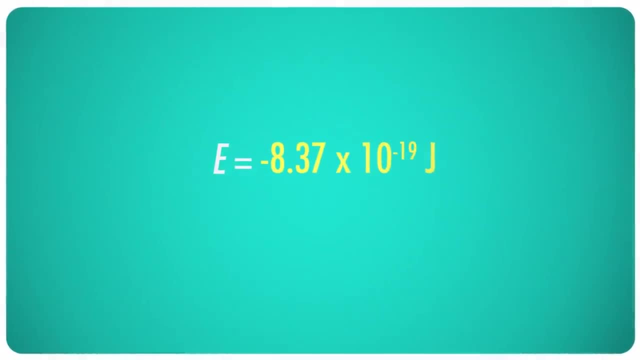 negative 8.37 times 10 to the negative 19th joules of energy. Remember that negative number represents a decrease in the energy of the system due to an attractive force. Remember that negative number represents a decrease in the energy of the system due to an attractive force. 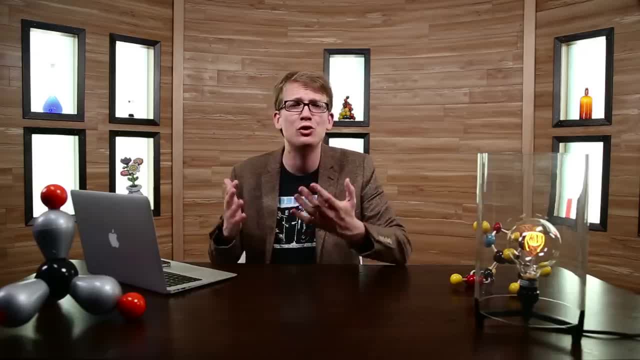 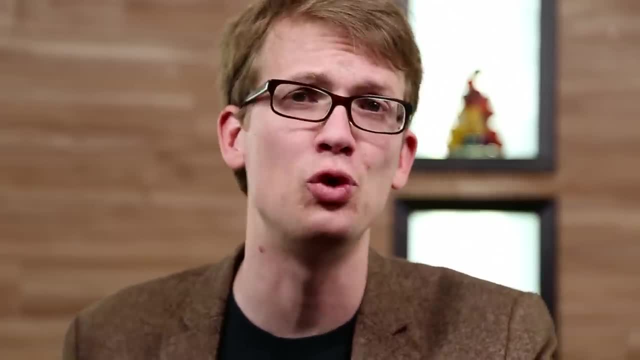 Which certainly makes sense here. Sodium and chloride ions are strongly attracted to each other due to their opposite charges. Of course, you might have noticed that negative 8.37 times 10 to the negative 19th joules looks like a tiny, tiny number, But keep in mind we're talking about one single pair. 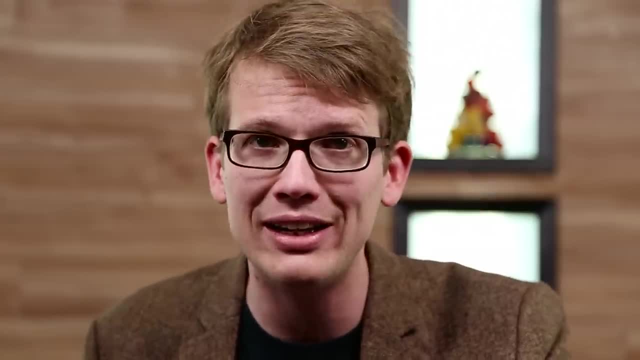 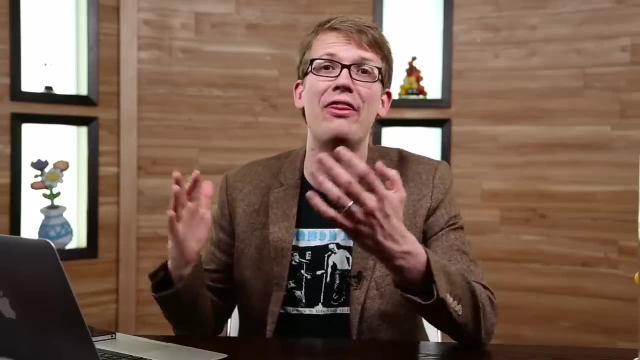 of ions, The negative 239 kilojoules that we got for chlorine. that was for a whole mole of molecules. When multiplied by the 10 to the 17th or so ions in a single grain of table salt and then by the thousands of grains of salt in a mole, the energy becomes. 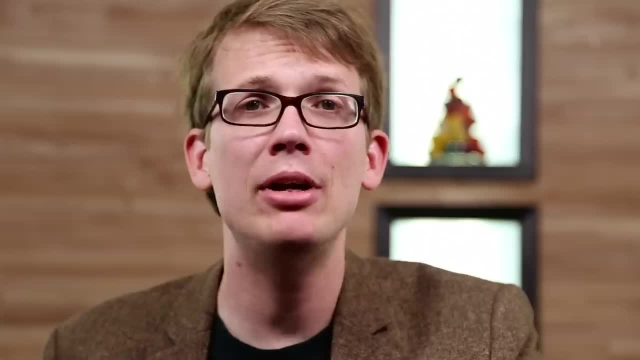 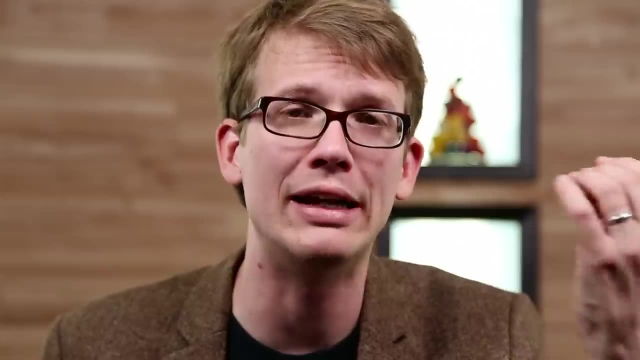 much more significant. The NaCl bond is in fact quite strong And because they consist of a positive ion and a negative ion, two charges completely separated between two different particles, Ionic bonds are extremely polar, Way more polar than polar covalent bonds. 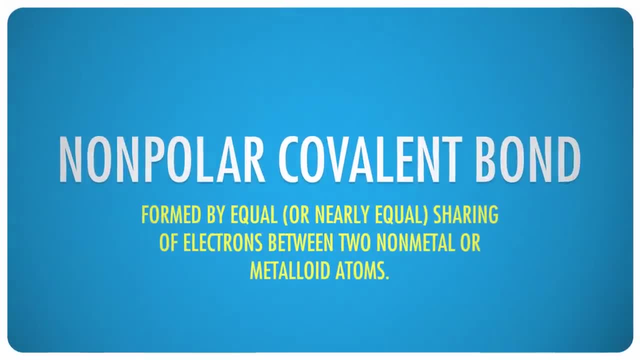 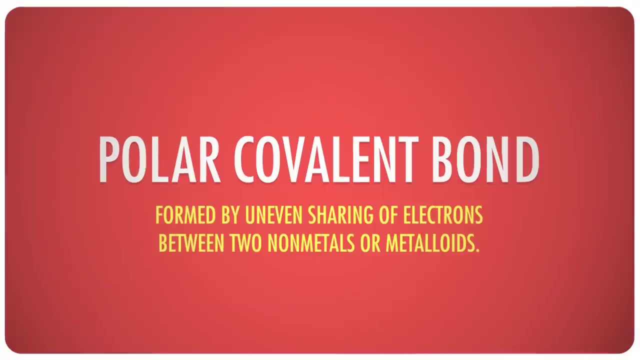 And so those are our three types of bonds: Nonpolar covalent, formed by the equal or nearly equal sharing of two electrons between nonmetal or metalloid atoms. Polar covalent, formed by the uneven sharing of electrons between two nonmetals or metalloids, And ionic. 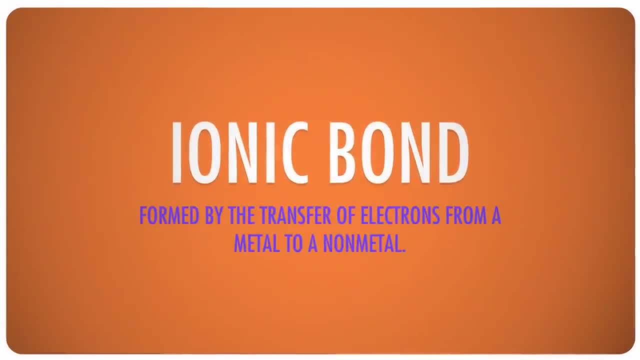 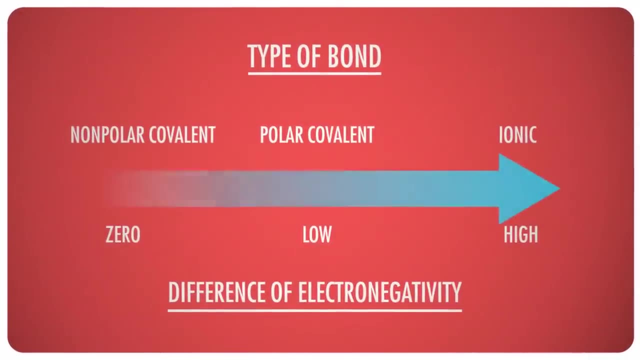 formed by the transfer of electrons from a metal to a nonmetal. It's important to remember, though, that there aren't only three designations for chemical bonds. Just like human relationships, bonds don't always have really well-defined boundaries. Everything is a continuum. Labels are useful, but they can only take us so far. 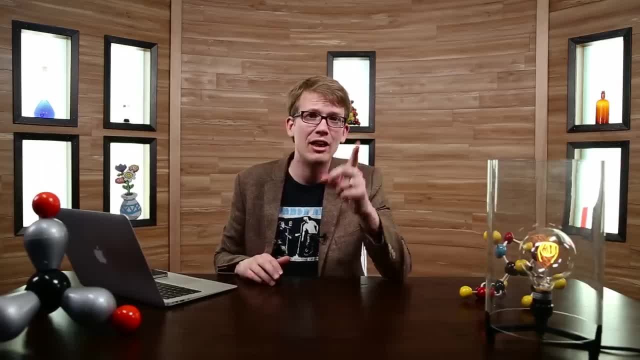 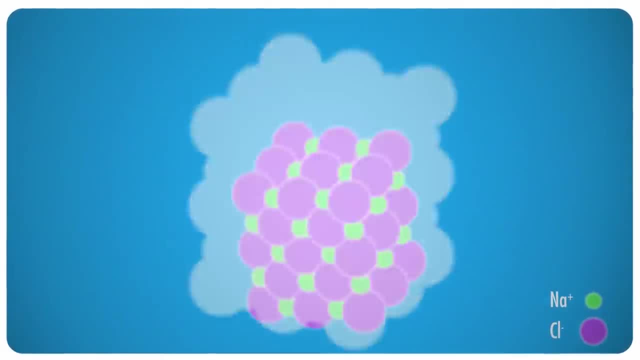 There are, however, certain properties that each kind of bond tends to have that you should know. For instance, ionic compounds are often crystalline in their solid form because of the way the ions pack together, like salt is. They're generally soluble in water because